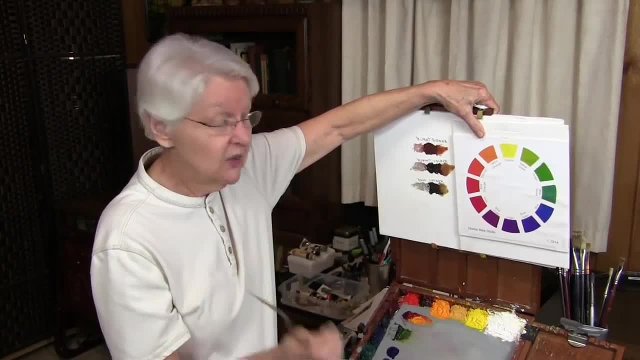 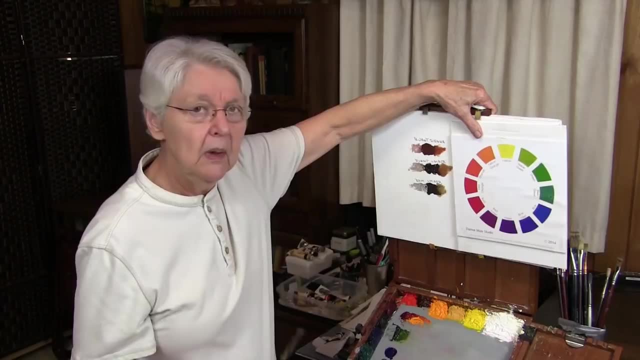 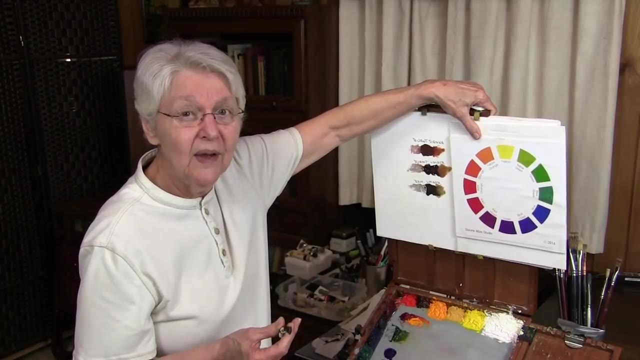 Remembering that color has hue value and intensity, And all three of these colors are dark value and they're very, very, very low in intensity. So how do we lower the intensity Of these hues? And we know the answer to that already: It's by adding their complement. So 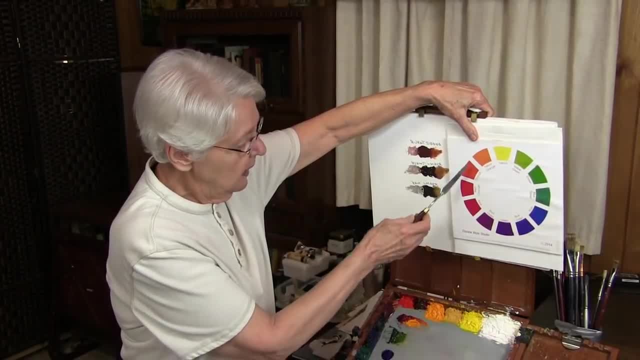 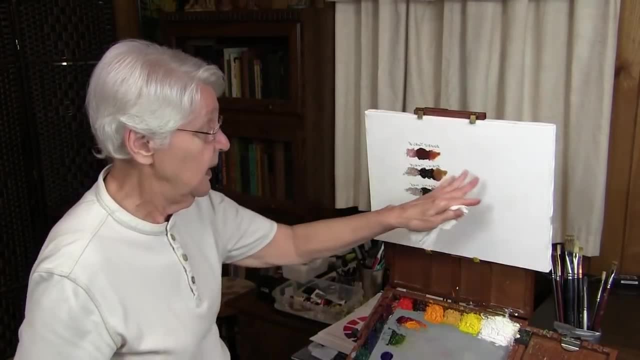 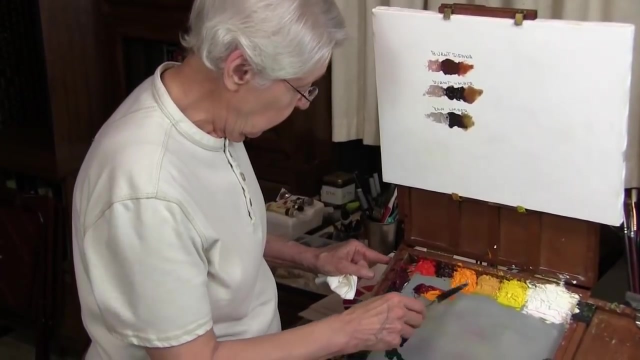 the orange, the red orange, which is burnt sienna. we would add blue, And let's just do that before I go on and show you how we get burnt sienna by adding orange and blue. So I'll come down to the palette here. Now I'm going to mix an orange here. I don't have an orange per se on my palette, but I 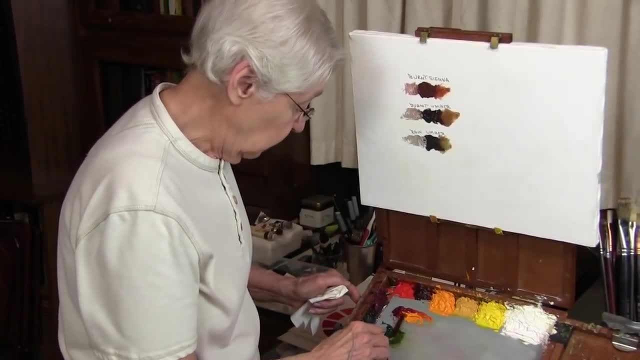 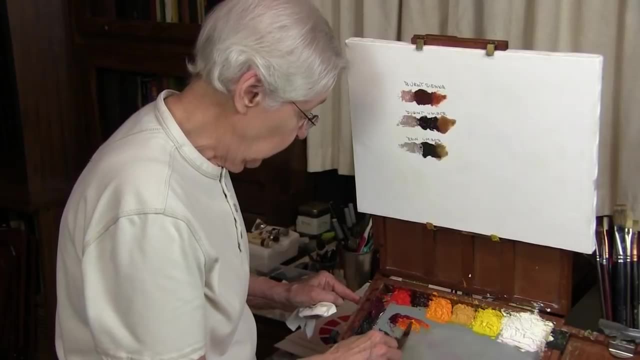 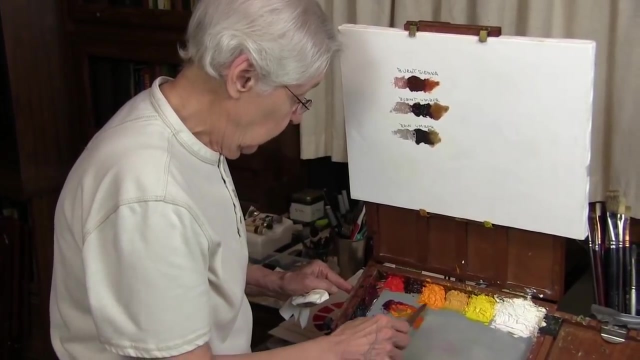 will create an orange. So I'm just going to mix alizarin crimson and the cadmium yellow deep. This is the cadmium yellow deep that's made by Rembrandt. I'm going to mix those to make an orange right here, Just like that. Now, you know, an orange can kind of fluctuate a little bit, It might appear. 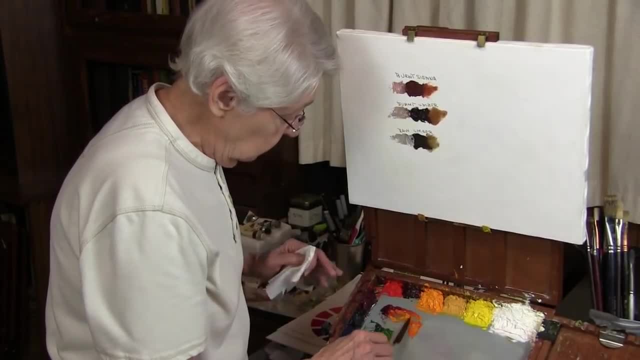 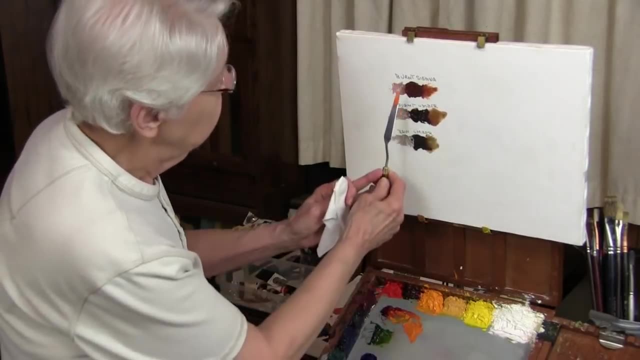 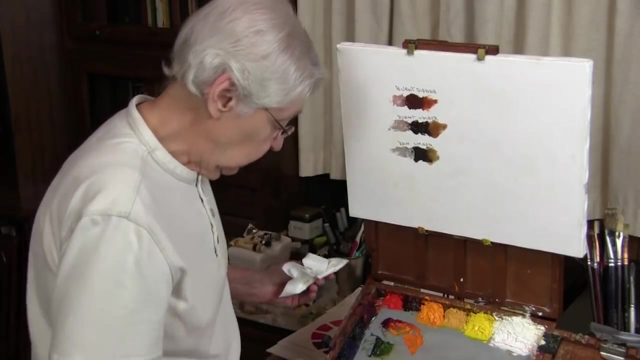 orange on, a little more towards red in some oranges and a little bit more towards yellow on others, But there's an orange. Now when I put this on the back of my palette and I can put it here, you see how very bright, intense that orange is. Now let's gradually add a little blue to that. 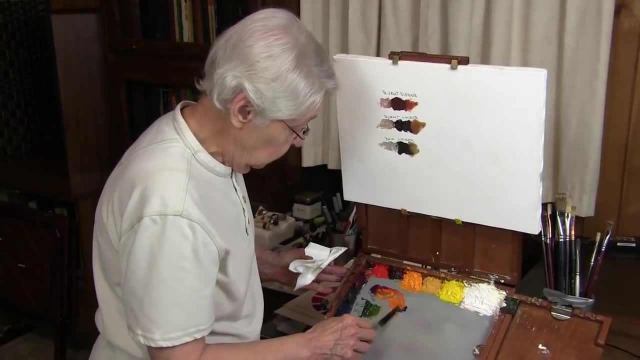 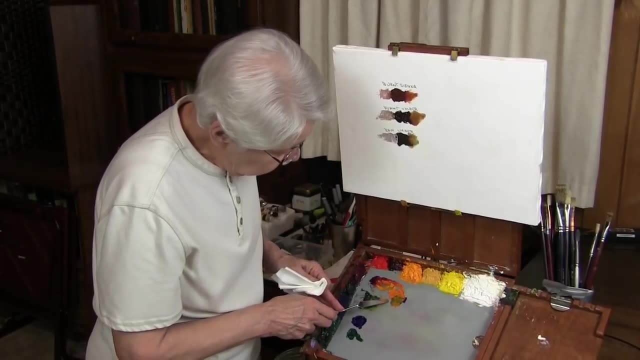 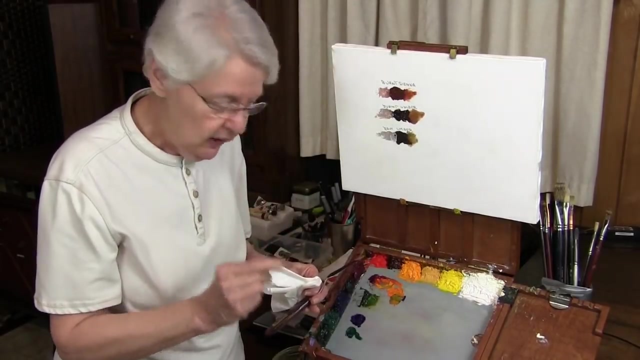 orange. I'll gradually add blue into this orange. Now when I do that- and here's a good clue for you- As I do that, as I begin to pull the blue into it, if it starts appearing green, then I know it doesn't have enough red. Red and green are complements, So I will have to pull a little bit. 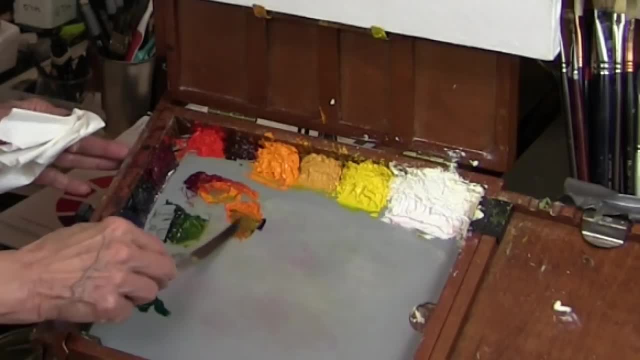 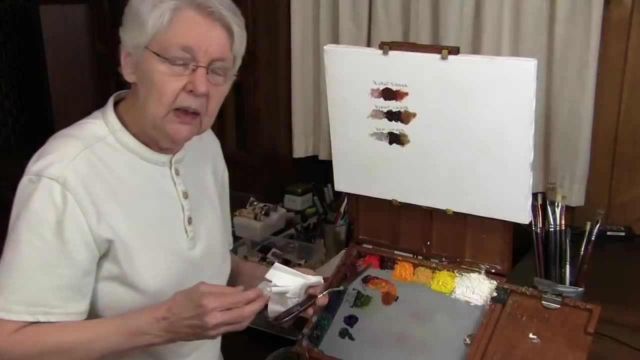 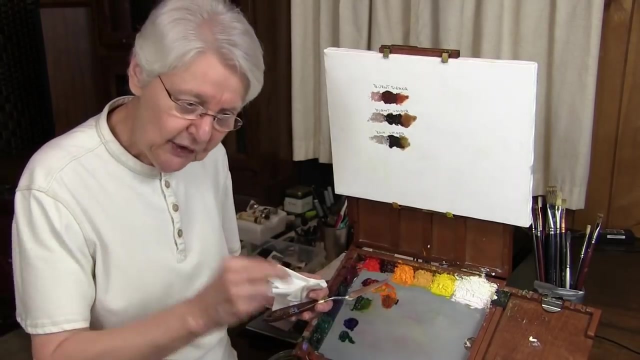 more red into that orange which I just did. There. we go right there A little bit more red. So it depends upon which orange you have. You can't just take any orange out of a tube, put it down, take any blue out of the tube and add to it and know that you're going to get burnt sienna. 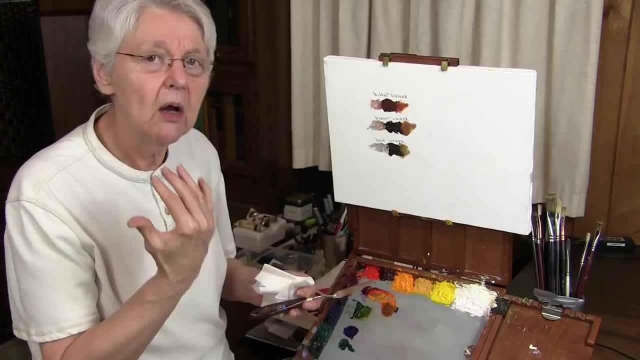 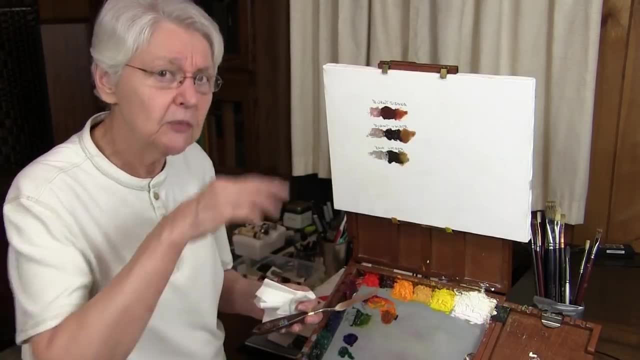 You adjust according to what you know how color works. So if an orange has more red in it, then it's going to to require. if an orange has more red in it, it's going to require a blue that has more green in it. 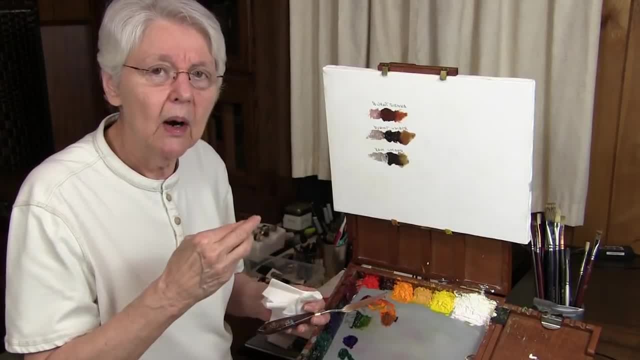 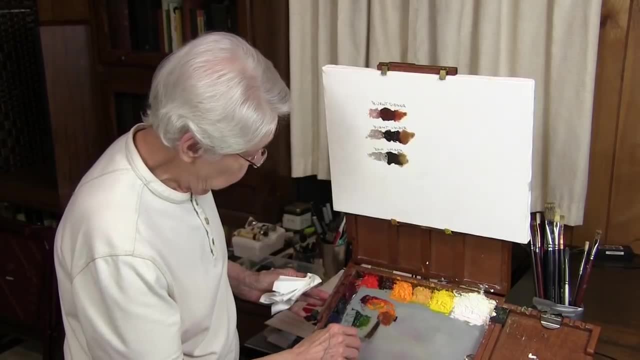 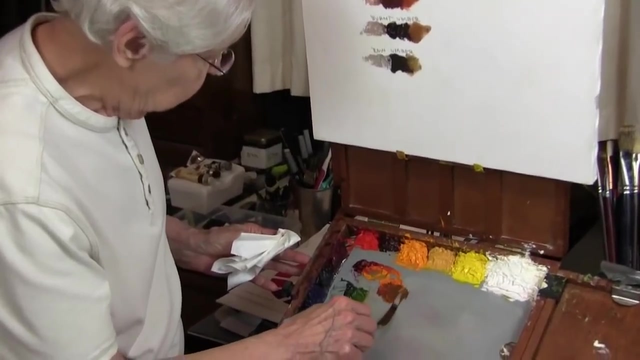 If the orange has more yellow in it, it's going to require a blue that leans a little bit more towards purple. So let's see what we've got here. Do we have a Brynsiana yet? Well, this is pretty close to Brynsiana. Put a little bit more blue into it. a little bit more blue, maybe just a touch. 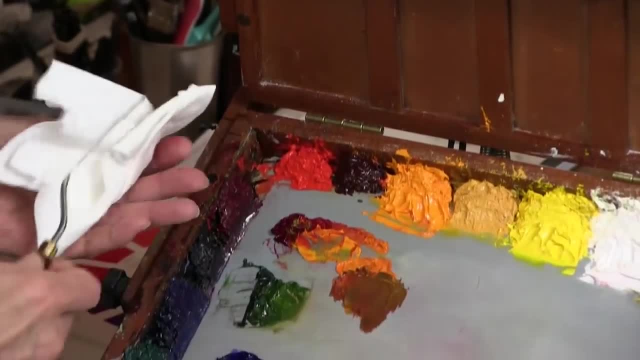 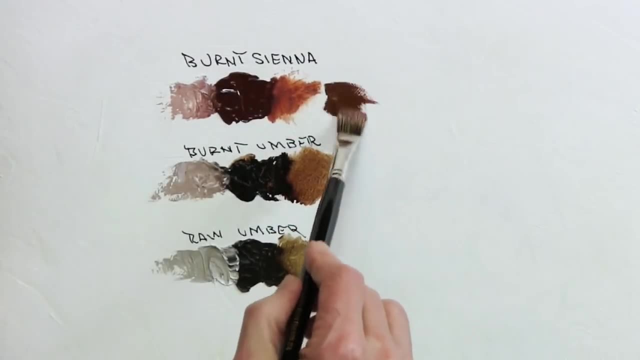 more and that looks pretty close to Brynsiana right there. Let's just take a brush and put it right here and you can see I'm pretty close to Brynsiana. Now what I've done with each one of these splotches of color here on the canvas. I've shown the color as it comes out of the tube. 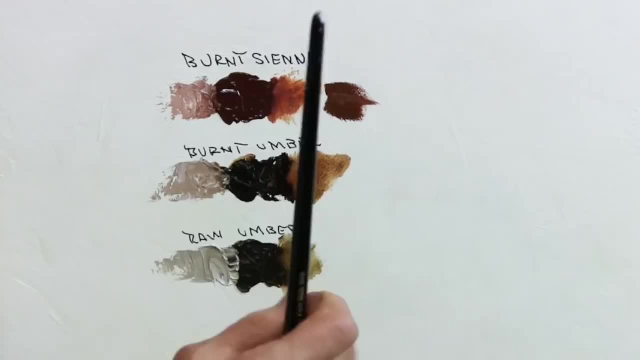 I've shown it thinned here with medium. This would be how it would behave if you're using it in a glaze, but also shows you pretty much what color it is. And then here I've mixed white with it. White always cools the color, so I've done that with each one of these colors. 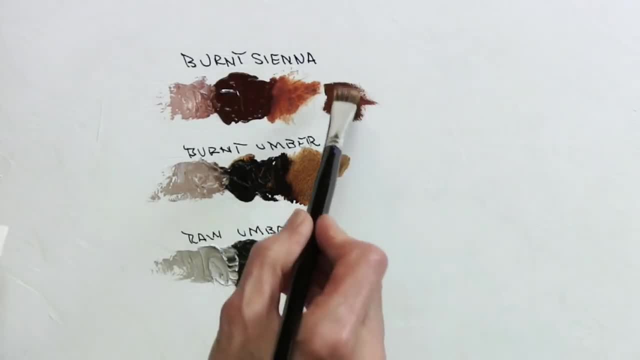 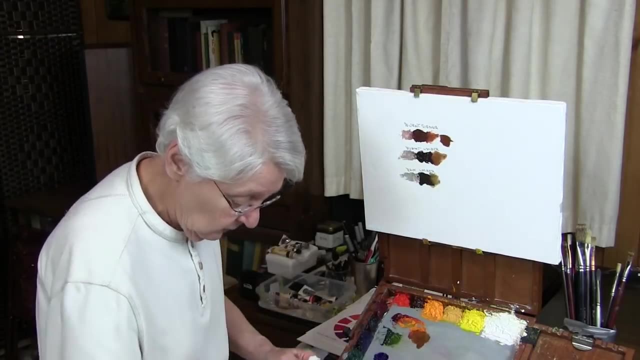 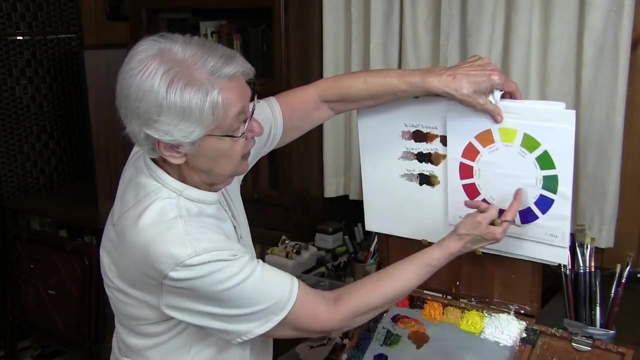 So you can see there that I've gotten pretty close already to mixing Brynsiana just by adding orange, mixing orange and blue. Now we'll go to the next step. and what do we do for burnt umber? So what we know about burnt umber is that it's more of a red-orange That tells me that we need. 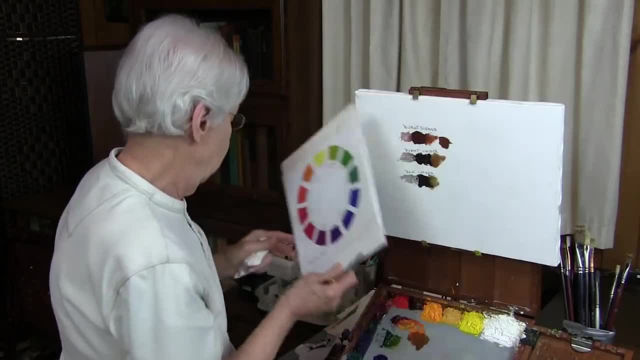 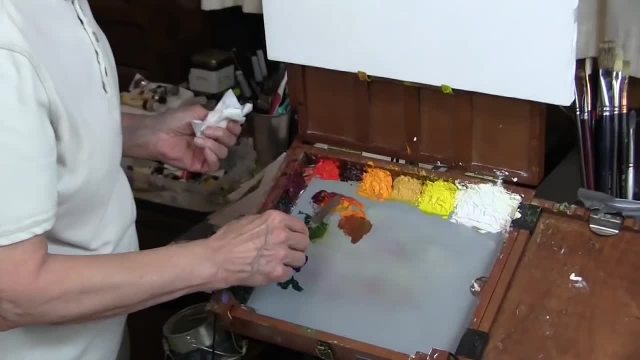 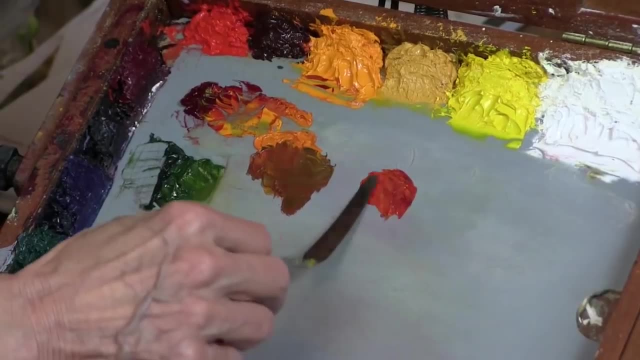 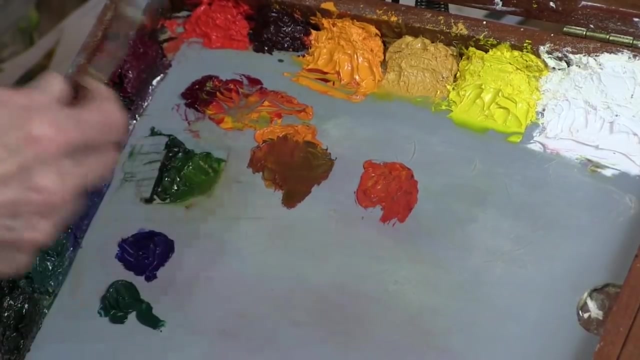 go back to this pile, and I'm going to go back to this pile and pull a red-orange mixture, one that leans more towards an orange that leans more towards red, rather than an orange that leans more towards what we recognize as the hue of orange. 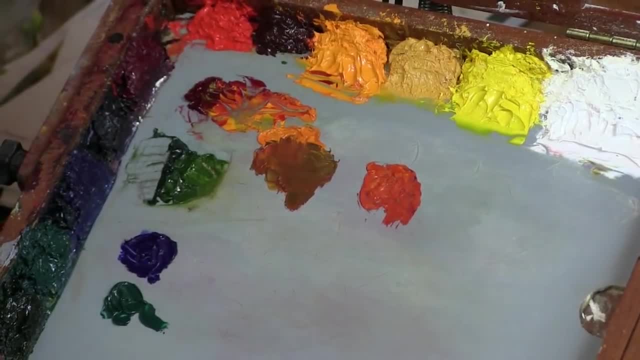 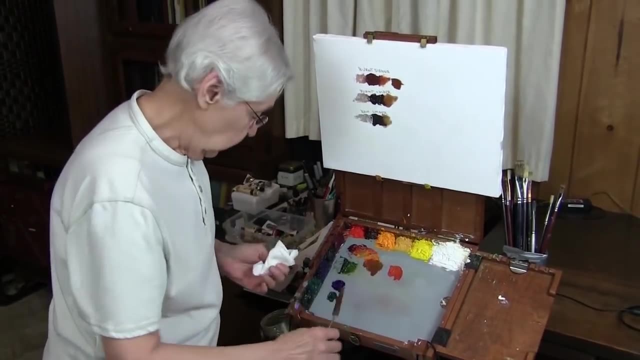 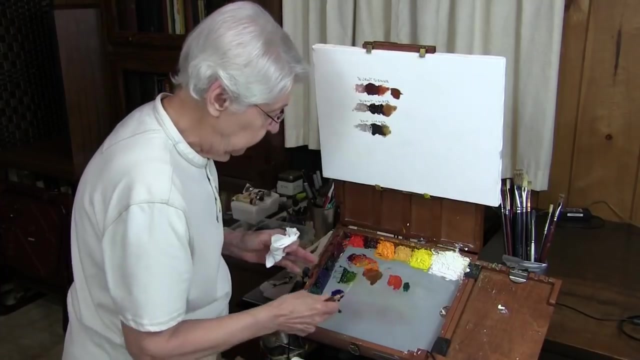 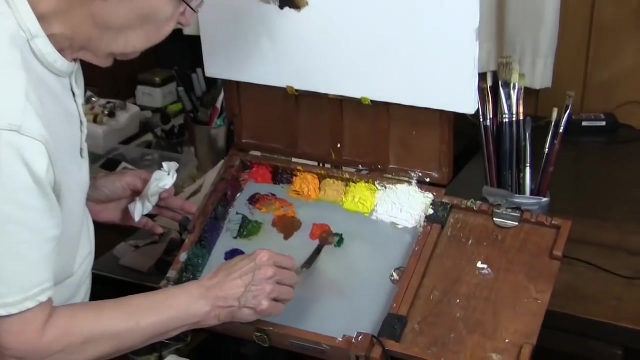 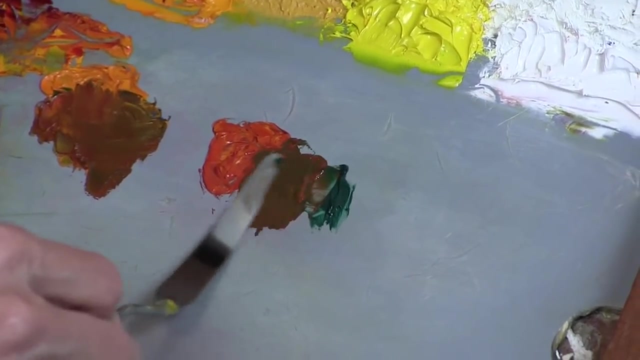 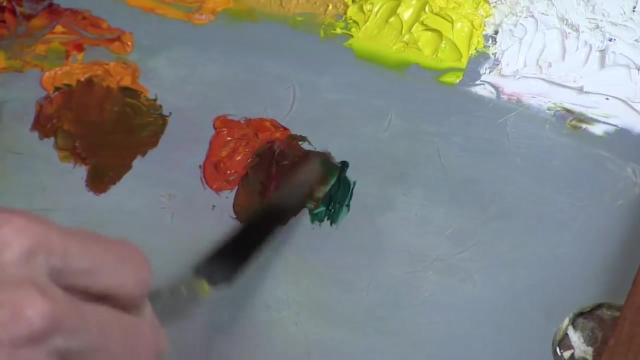 Now I have a Rembrandt Faridian which I've done a YouTube quick tip about, and that's a nice blue-green, The Rembrandt Faridian. so I'm just going to go ahead and go for it and we'll just take the Rembrandt Faridian Now, gradually pull Rembrandt Faridian into the red-orange and we're already getting very close to burnt umber Right in there, very, very close to burnt umber. I probably could stand a little bit more red, so I'm going to add a little bit of the alizarin back into that and I'm going to go ahead and go for it. 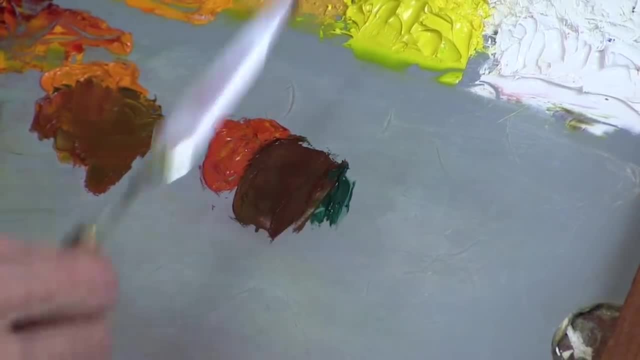 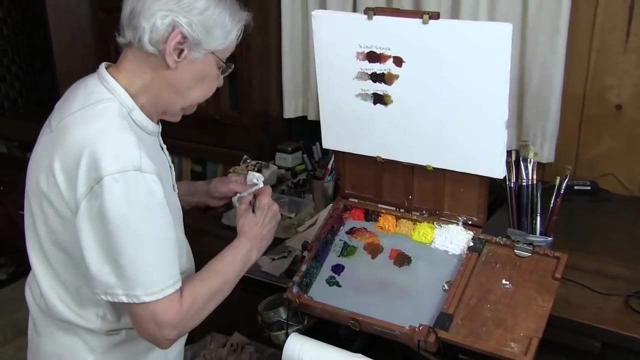 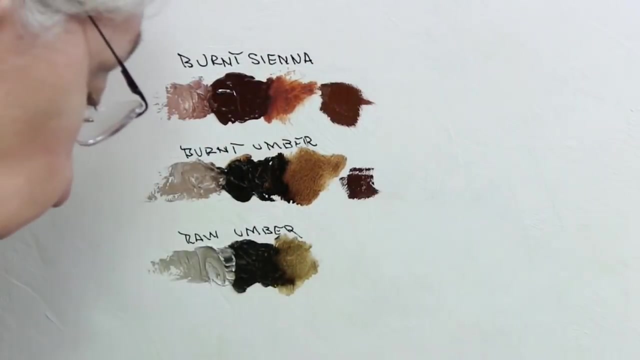 So we see that that red-orange is a little bit redder than I had thought it was. So that gives us pretty close to burnt umber. So we'll just put burnt umber right here or my mixture that's very close to burnt umber right there. 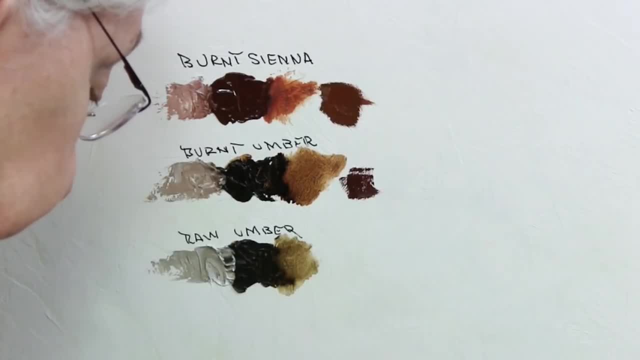 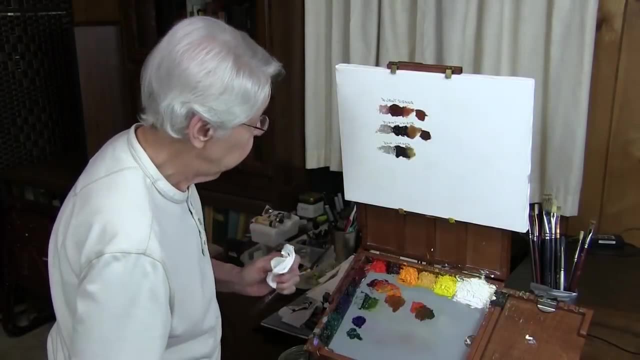 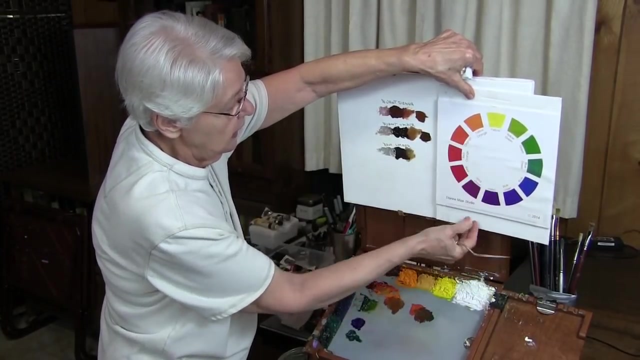 There we go. It's very, very close to burnt umber. Now for raw umber, Now for raw umber. as it appears on the color wheel, the hue of raw umber is more yellow-orange. So that would tell us. 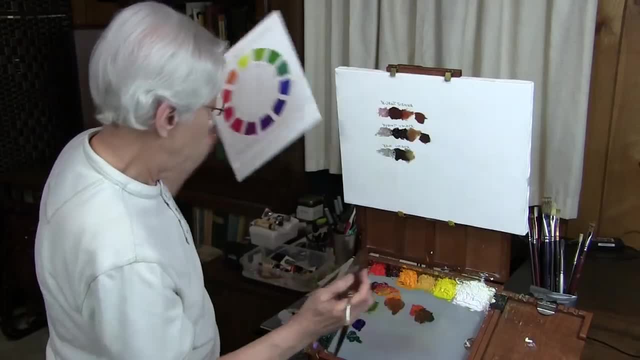 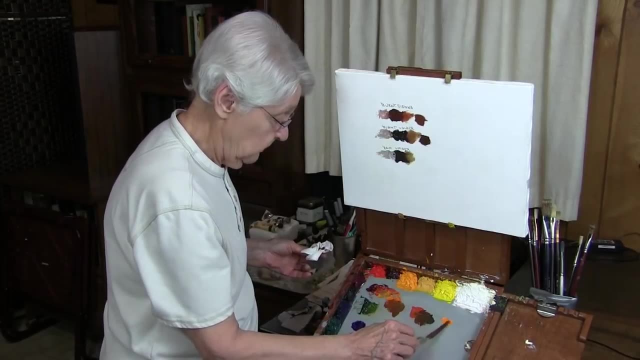 if it's more yellow-orange, it tells us that we need more of a blue-violet, tells us that we need more of a blue-violet. So if I start out with yellow-orange- Now, this is yellow-orange, right here It may. 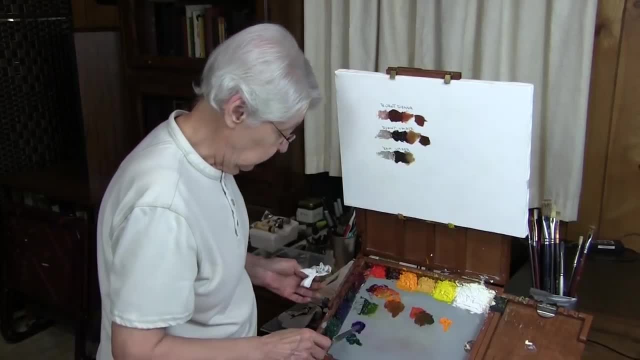 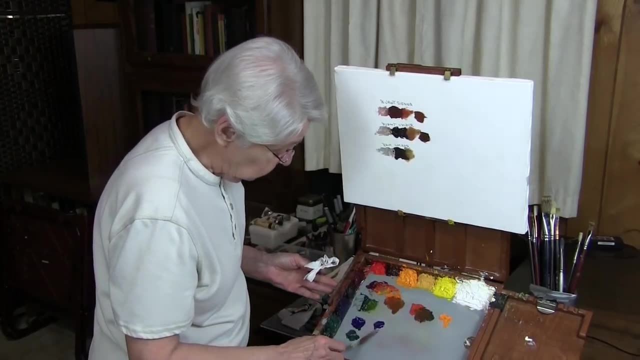 be a yellow-orange. that needs to become a little bit more orange, but we'll find out in just a moment. Now I can take the ultramarine blue, add a little bit of oddly viridian to it and I get a blue-violet. 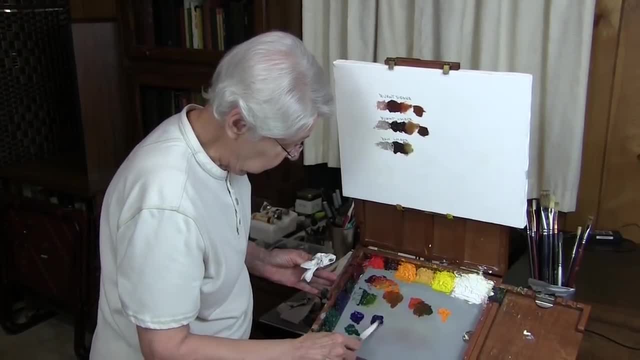 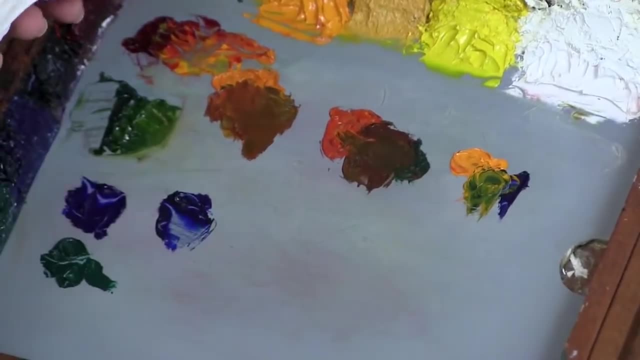 Now, of course, these things may have to be adjusted, but this is what we start with. Okay, I start pulling the blue-violet into the red orange. I see it turns green. so what does that tell me? It tells me I don't have. 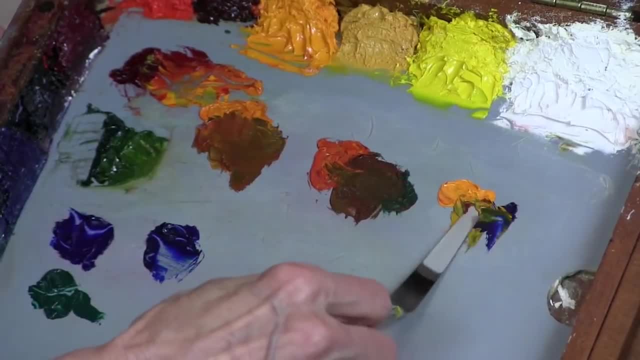 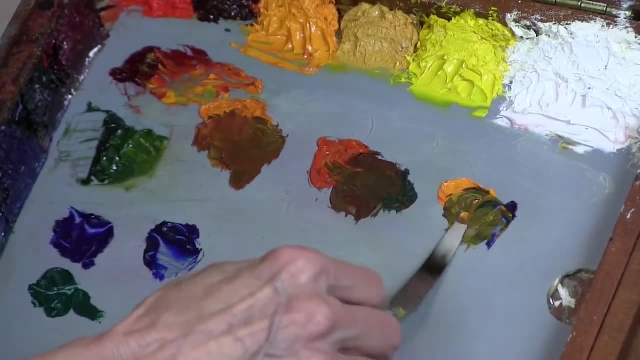 quite enough red, so I add the red back in, Get the blue-violet going, add the red back in and I should be able to find raw umber. It's still a little bit on the green side, so it means that red-orange. 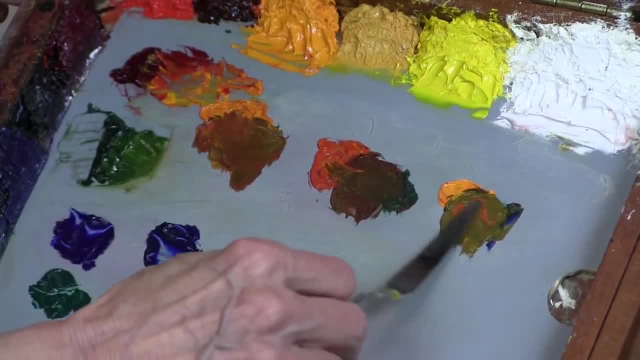 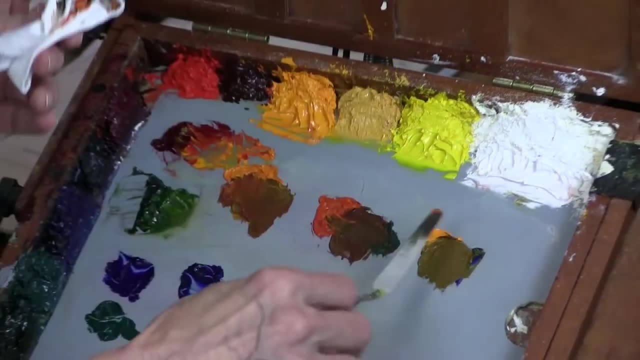 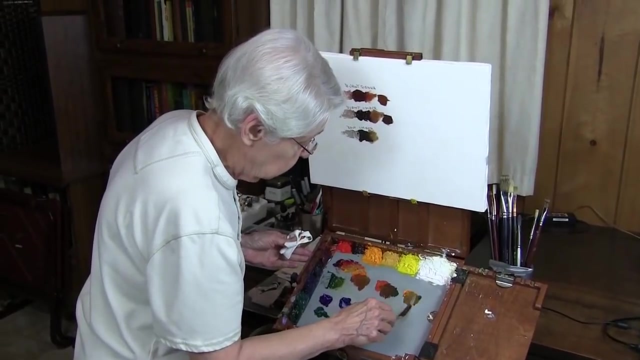 actually registers a little bit more red than it does. orange- See how's that for raw? That's pretty close to raw umber Right there And just a little bit more here. Get that just a little bit more adjusted to to uh. 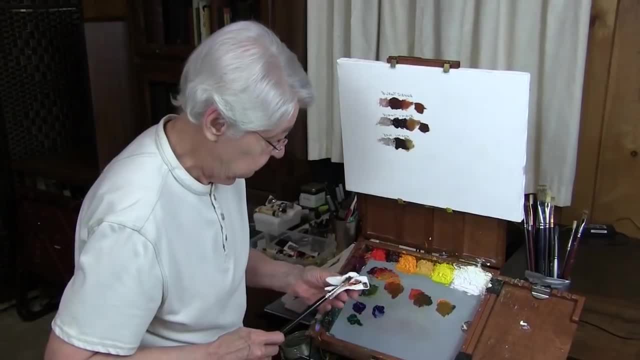 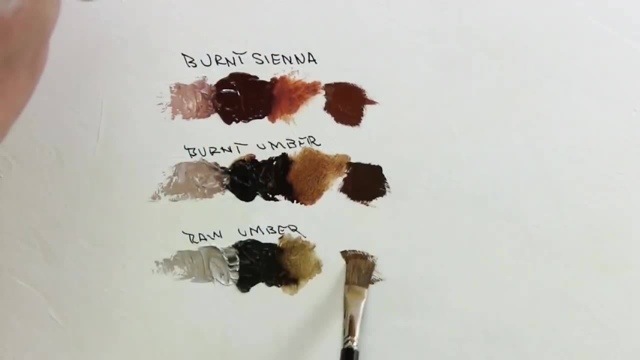 yeah, that's pretty close to raw umber, So I will pull that one out So you can play with these colors. It's fun to play with color And it's fun for me right in there. That's, uh, very, very close. It's.